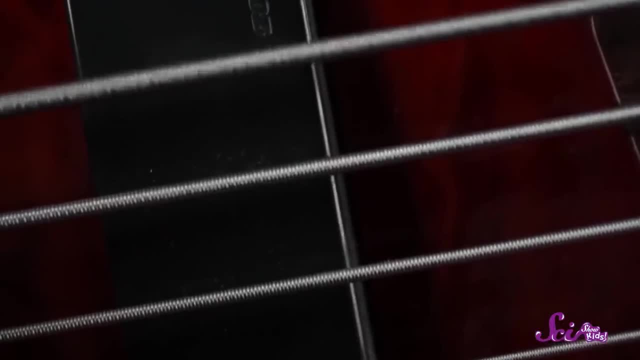 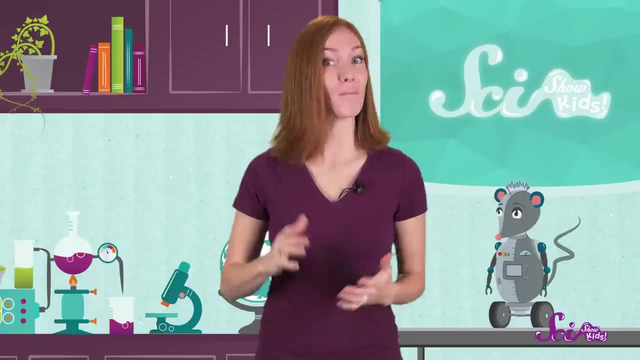 Can you see the string of the guitar moving really fast? That's a sound just getting started. Now, after something like a vocal cord or a guitar string moves, it makes the entire sound move. It makes the air move too, And we know that air is made up of very tiny particles, and these particles end up carrying 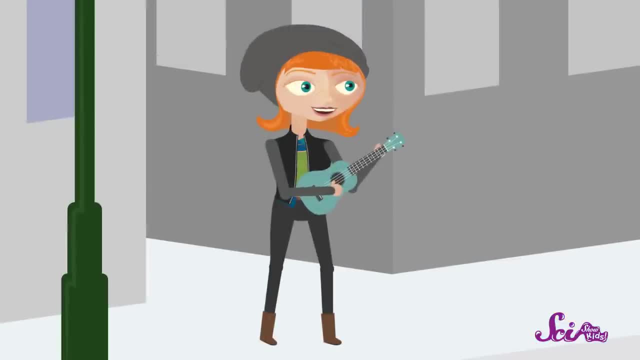 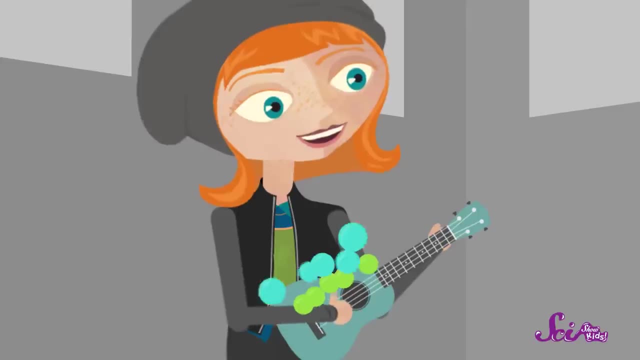 the vibrations through the air, so sound can travel. For example, when a guitar string moves, the particles in the air around the string start to move too And then they bump into other particles, making those move. These particles carry the vibrations through the air until it hits your ear and you can. hear the music. But the problem is the vibration starts to go away pretty quickly After traveling through the air for a bit, the particles don't bump into each other as hard and eventually the vibration stops. And if that happens before the vibration makes it to your ears, you don't hear anything. 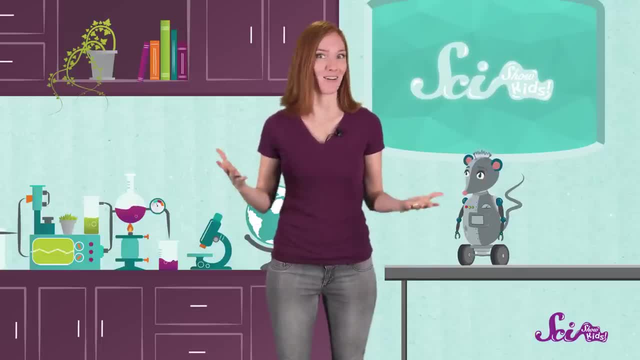 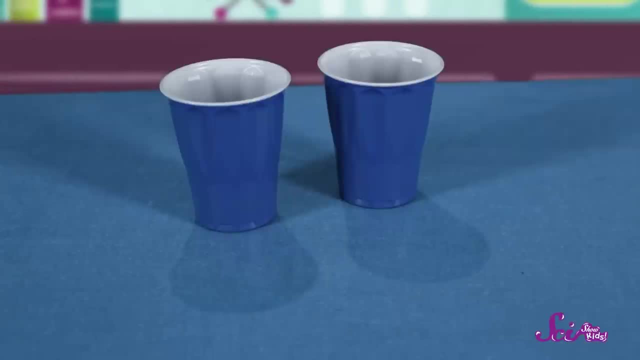 So now we know that vibrations can make the air move to produce sound, Do you think they can make other stuff move too? Let's try it out. You'll need a grown-up, two paper or plastic cups, a bit of tape, a sharp pencil or a pair. 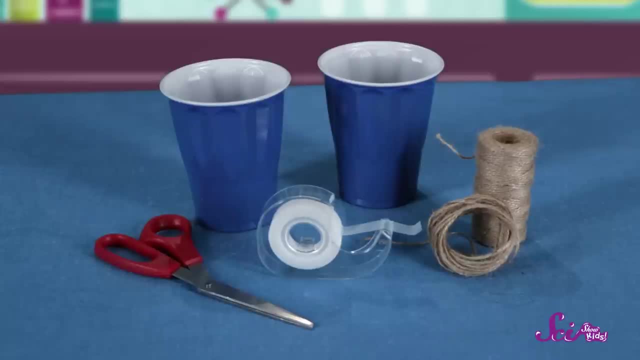 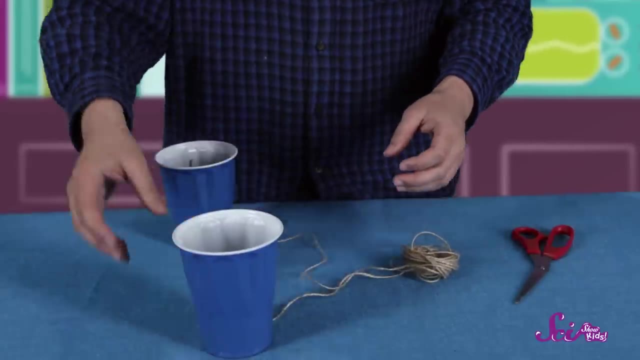 of scissors and a long piece of string, say three to nine meters long. Use the scissors to poke holes in the bottom of each cup. Now thread the string through each hole so that the cups are facing away from each other. If you can, tie a knot at the end of each string inside the cup. 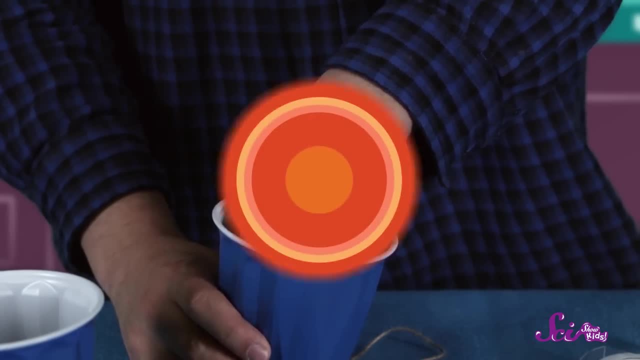 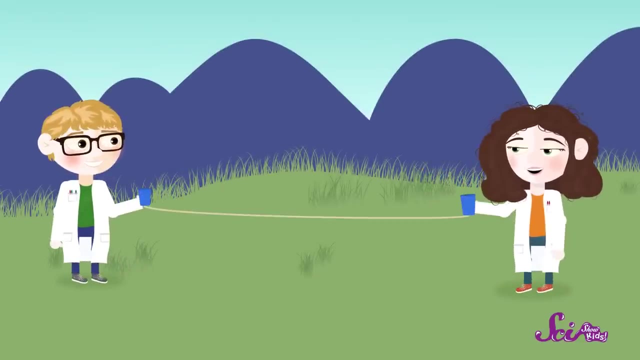 You can put a little bit of tape on the string too, just to make sure it doesn't come out. Now give one of the cups to a friend and take one for yourself. Walk away from each other slowly until the string is in a straight line between the two. 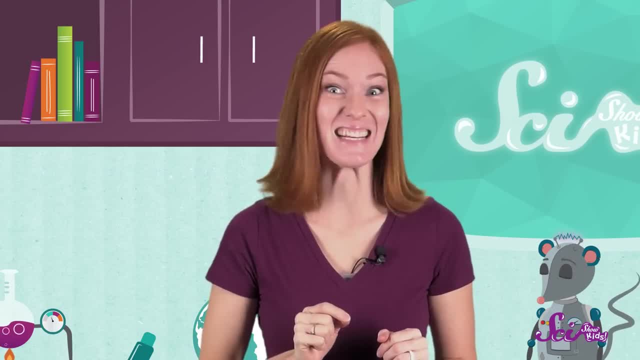 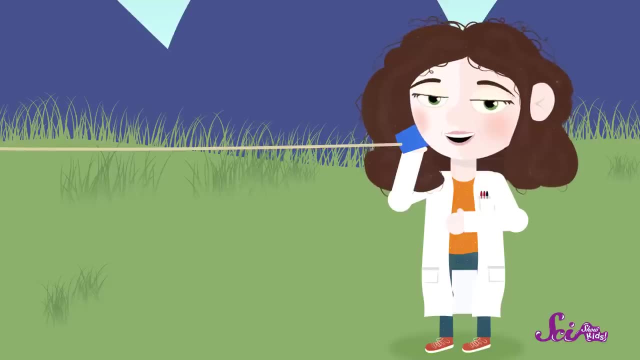 cups- And this is important- Make sure the string is tight. Now tell your friend to put their cup over their ear. While you talk into your cup, Can your friend hear you? Now try putting the cup over your ear and give your friend a turn to talk. 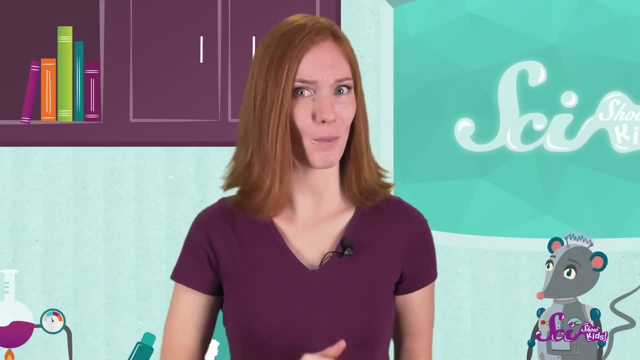 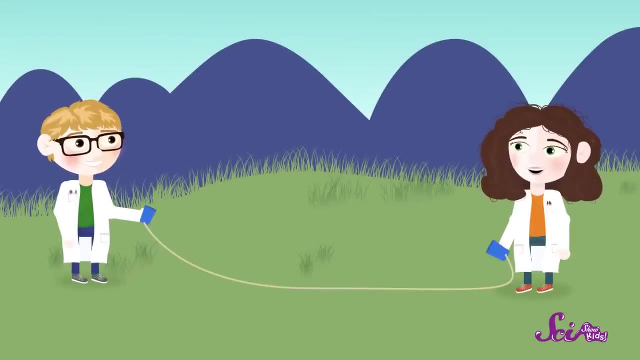 Can you hear them? Pretty cool, huh. Are the cup and string helping us here? Let's do a test: If you keep your voice at the same level and try to talk to your friend without the cups, can they hear you? 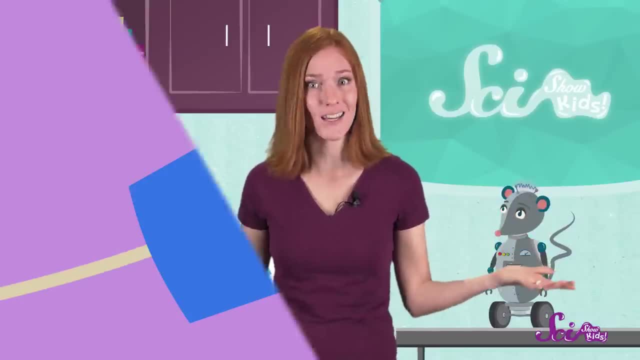 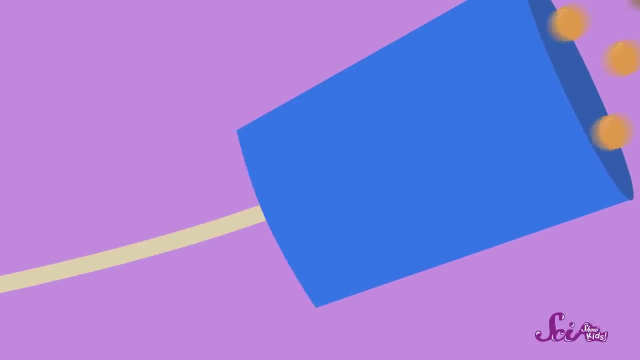 Well, yes, But not as well. So what's going on here? When you use the string phone, your voice makes the air particles in the cup start to vibrate. These vibrations then make the bottom of the cup vibrate, See.